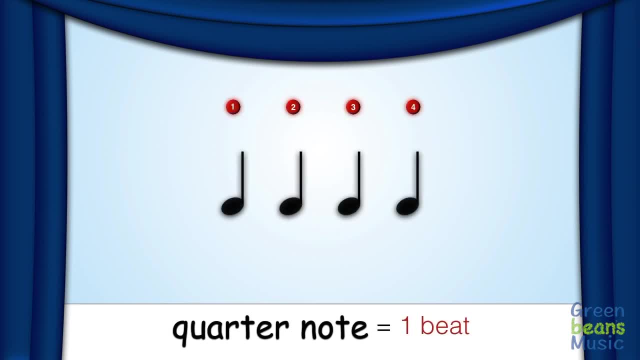 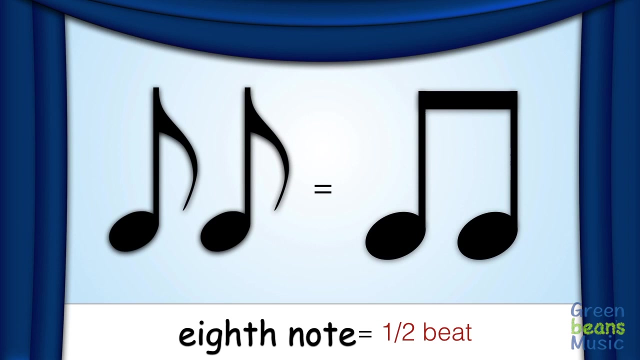 Each quarter note gets one beat. Since we have four beats, we'll use four quarter notes. The eighth note: The eighth note has a shaded in note head, a stem and a flag. Eighth notes can be written individually with a flag or connected with a beat. 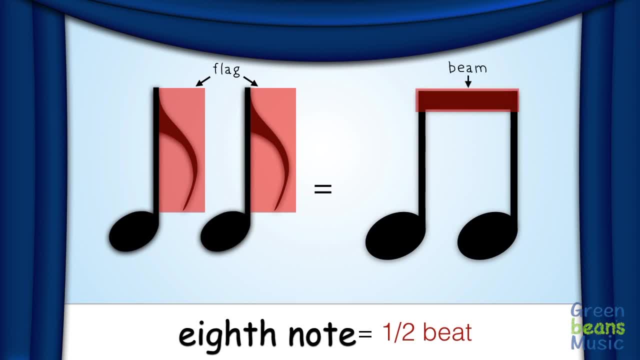 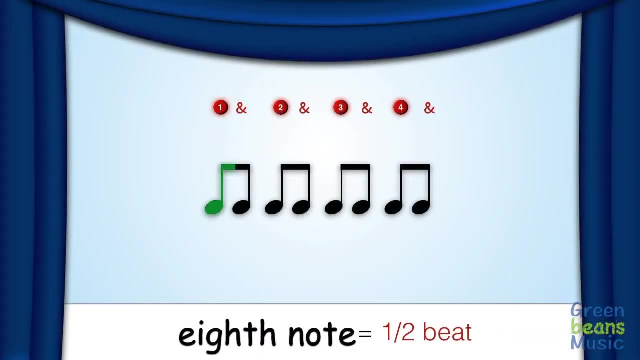 Eighth notes can be written individually, with a flag or connected with a beat. Eighth notes can be written individually with a flag or connected with a beam. The eighth note equals half of a beat. You try Last time. The sixteenth note Has a shaded in note head stem and two flags. 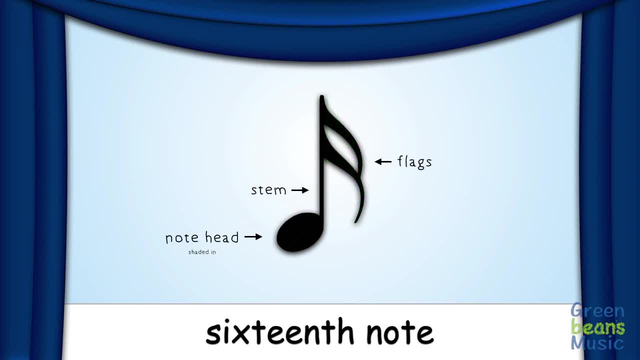 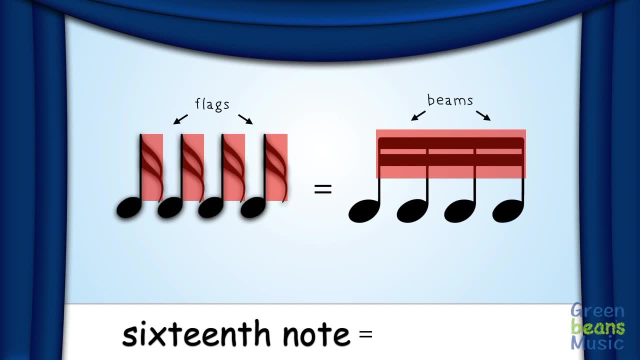 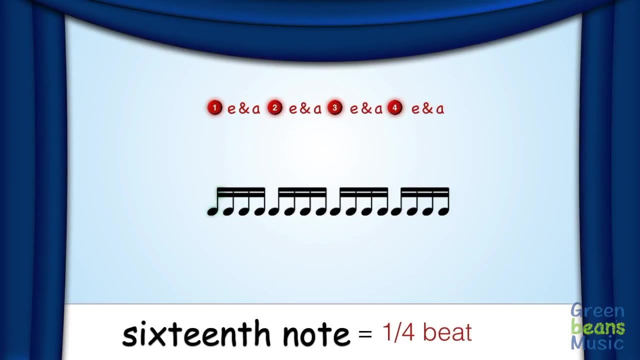 The flags are how we tell the sixteenth note from the eighth note. Sixteenth notes can be written individually with two flags or connected with two beams. The sixteenth note equals a quarter of a beat. Eighth notes can be written individually with a flag or connected with a beam. 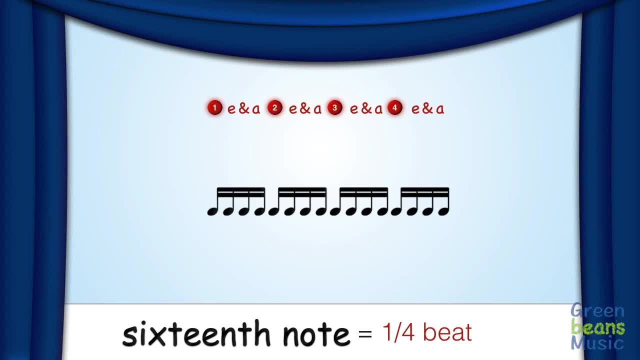 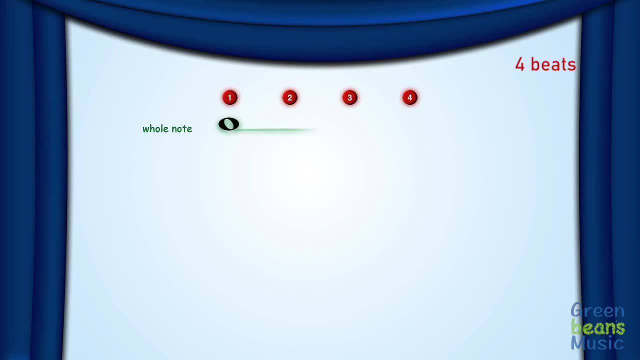 Eighth notes can be written individually with a flag or connected with two beams. Now let's review. The whole note gets four beats, The half note gets two beats, The quarter note gets one beat, The eighth note gets a half beat And the sixteenth note gets a quarter beat. 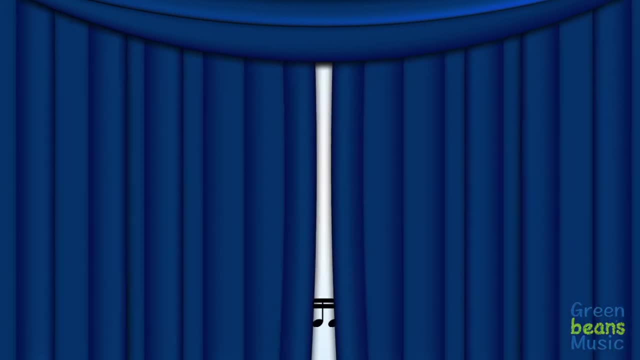 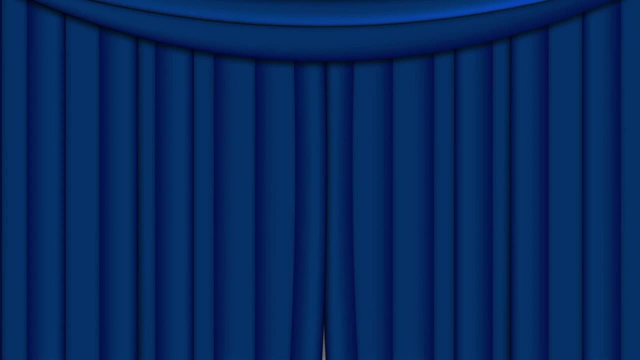